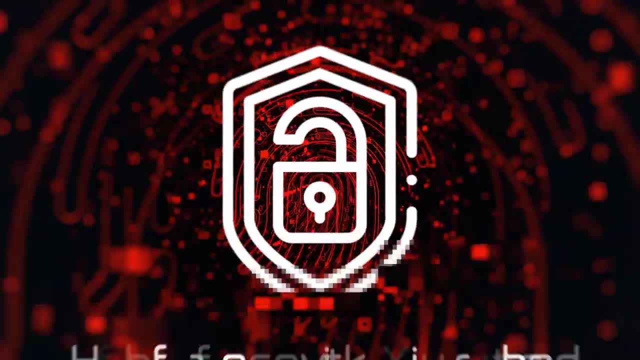 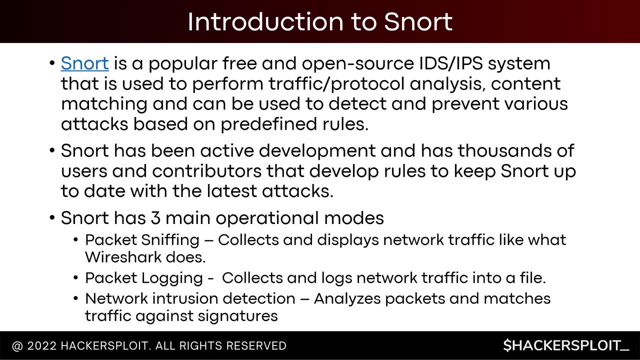 So what is SNORT? right, Because I've thrown around the term or the word SNORT quite a bit. SNORT is a popular, free and open source IDS IPS system, so intrusion detection system and intrusion prevention system that is used to perform traffic or protocol analysis content. 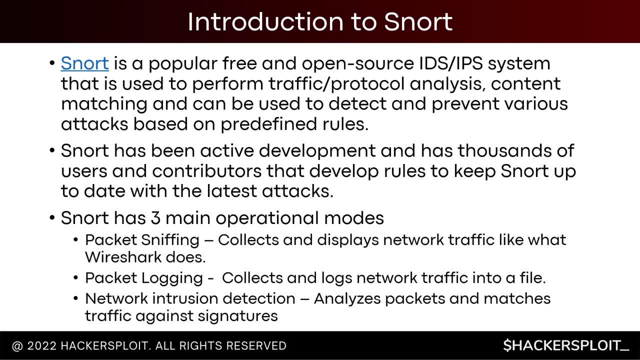 matching and can be used to detect and prevent various attacks based on predefined rules. SNORT has been in active development and has thousands of users and contributors that develop rules or rule sets to keep SNORT up to date with the latest attacks or the latest intrusions. 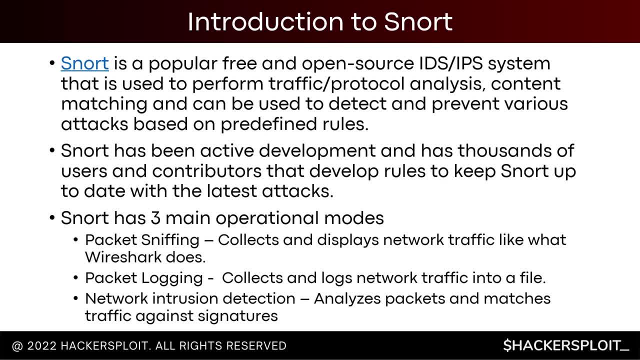 So the way I want you to think of a rule- because I've mentioned rules quite a bit here- is: you know, if you take a look at a firewall, you know a rule is essentially that It's just a rule that specifies what to do with a specific packet or with traffic from a specific port. 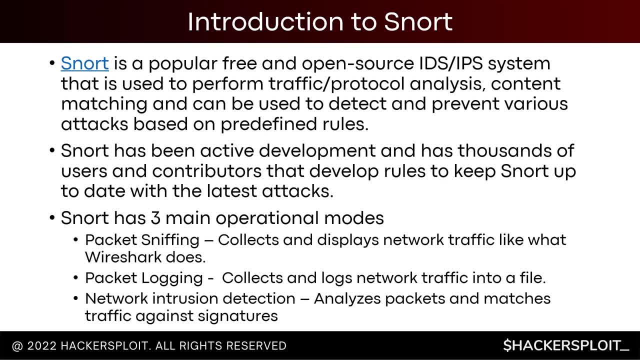 et cetera. And it's the same thing for SNORT, whereby you have the ability to, at a very basic level, log or essentially notify or alert individuals of specific traffic. So you know, I can notify the administrators or the security analysts that there is an FTP connection for. 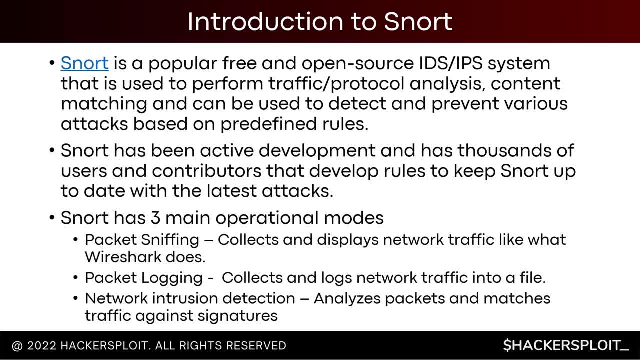 example. So one of the things with SNORT rules is you have the ability to perform signature matching whereby, based on the content contained within the packet, I can identify a signature and I can then utilize that signature to detect an intrusion or an attack. And I'll give you a practical example of 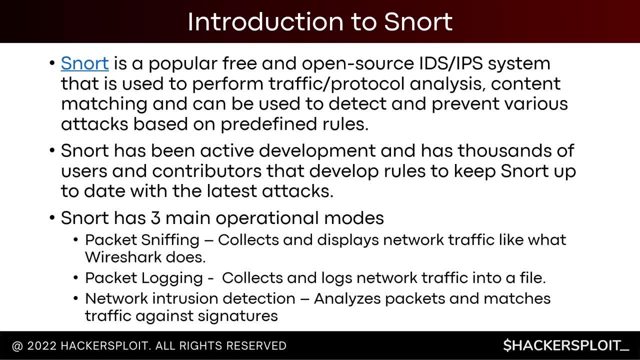 this during the practical demonstration. All right Now, in order to understand how SNORT works, you need to know that it has three main operational modes. All right, So you have packet sniffing, where it collects and displays network traffic, like what wires are connected to the network. 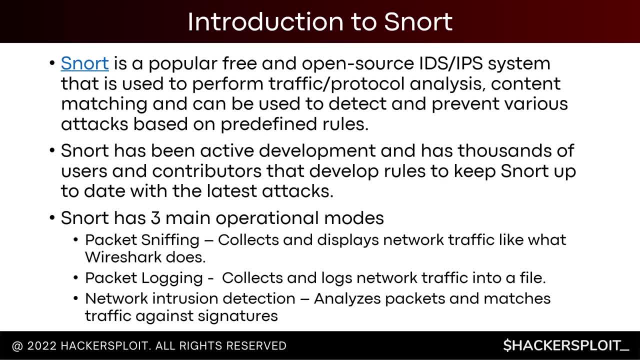 And then you have packet sniffing, where it collects and displays network traffic, like what wires are connected to the network. That's fairly simple. We can do that with Wireshark. We then have packet logging, which collects and logs network traffic into a file. Again, Wireshark also does that, And that's why I actually covered. 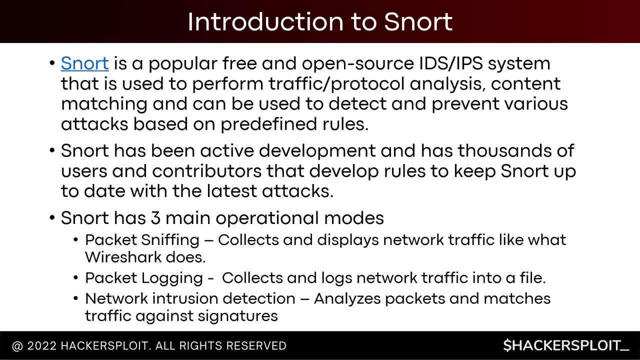 Wireshark to begin with, because we will be using it to actually analyze the logged traffic. But what we're focused on is the network intrusion detection operation mode that analyzes packets and matches traffic against signatures specified within rules or matches traffic against the rules that you have specified. 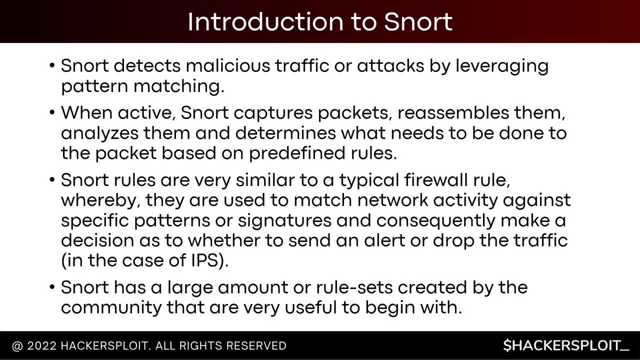 Now SNORT detects malicious traffic or attacks by leveraging pattern matching. When active SNORT captures packets, reassembles them, analyzes them and determines what needs to be done to the packet based on the on predefined rules. So if you install and configure SNORT but don't, and you know you disable the default community rules. 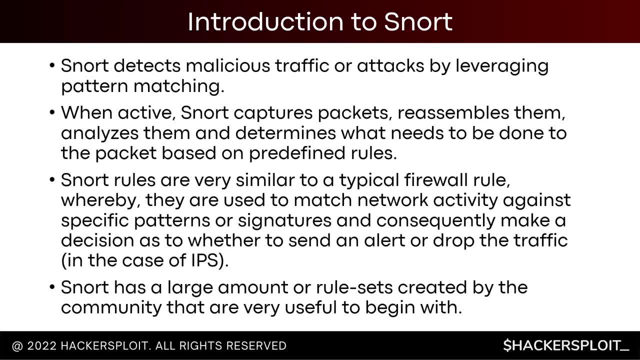 and you don't have any of your own predefined rules, then you know SNORT is pretty much non functional at that At that point. so what? the message I'm trying to convey here is that rules are. you know, the core are. 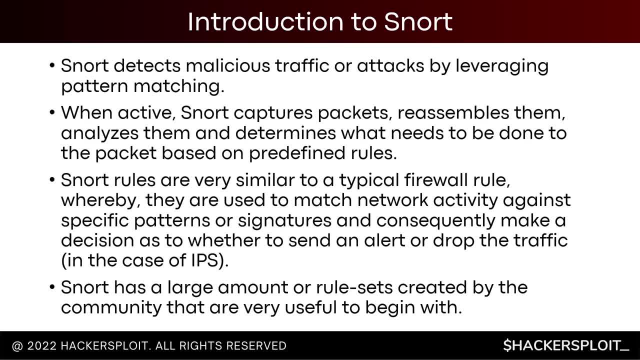 at the core of. you know the functionality of SNORT, So SNORT rules are very similar to a typical firewall rule, whereby they are used to match network activity against specific patterns or signatures and consequently make a decision as to whether to send an alert or drop the traffic in the 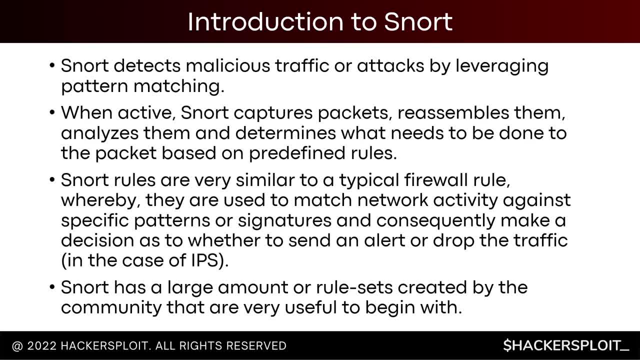 case of the intrusion prevention system mode Right now. one of the great things about SNORT that it has a large amount of rule sets created by the community that are very useful to begin with. now, why are these important? well, they're important because the community essentially 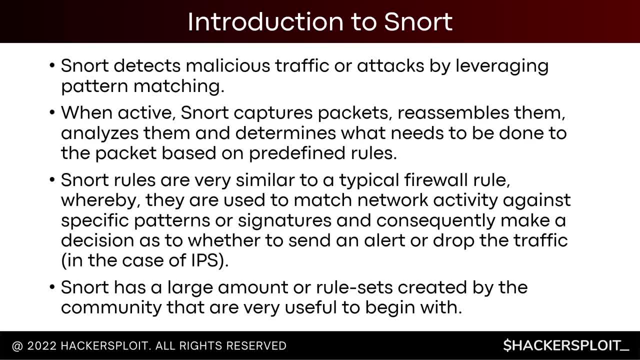 generates rules for the latest attacks or exploits, so that if you get the latest rule set, then that means that your network is up to date in regards to detecting these new types of attacks or intrusions, which is absolutely fantastic. now, another great thing with snort is that the, the, 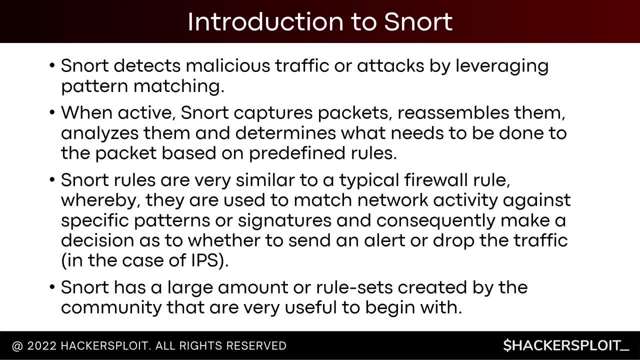 actual process of writing rules is extremely easy to understand and to actually do yourself. which means if you are a security analyst and there is a new exploit developed, you can essentially perform an analysis on that exploit and generate your own uh, your own uh snot rule to detect that, in the event that attack is performed on your network or the network that 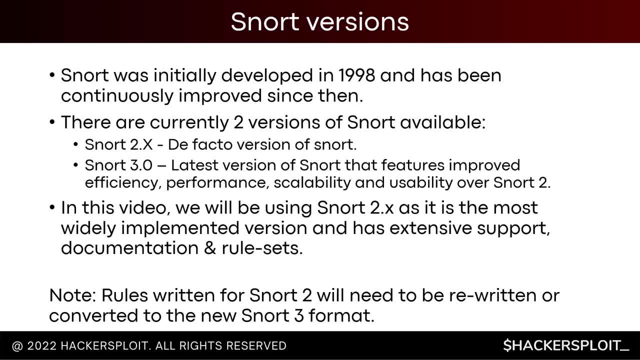 you're actually protecting. so let's talk a little bit about about the snot versions, because i think this is very, very important and there could be a confusion- uh, you know with what version to use. all right, so one thing to note is that snot was initially developed in 1998 and has been continuously. 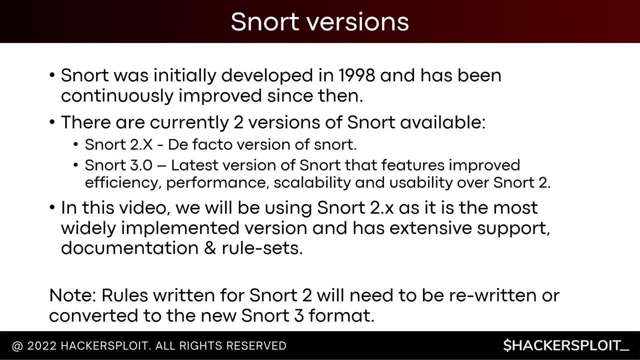 improved since then. what does that mean? it means that snot has been a an ongoing open source project and it has had a lot of contributions. and, of course, given the fact that it is open source, the typical release, the actual mode of release that they've utilized, is a. 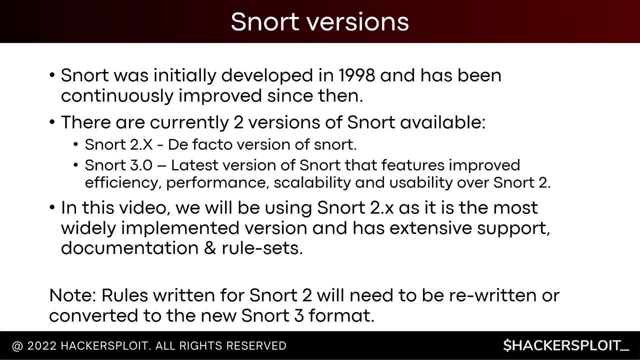 versioning system- that in in my case makes a lot of sense- whereby, you know, we currently have two versions of snot available. we have snot version 2.x, so that means you know whatever version of version 2, because there are many variants, but ideally you want to use the latest version of. 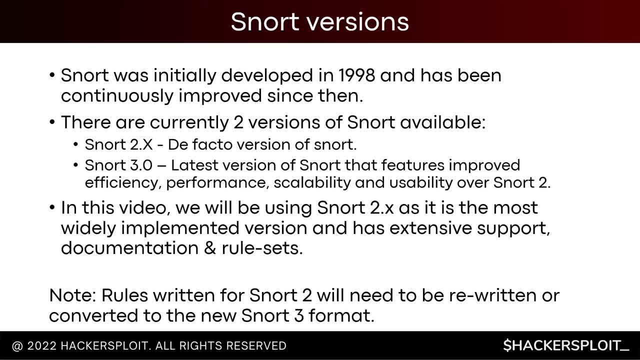 version 2.. so version 2 is the de facto version of snot and is the version of snot that is typically deployed or is most widely implemented and has the most rules or rule sets for snot. and then we have snot 3.0, which is the latest version of snot that features improved 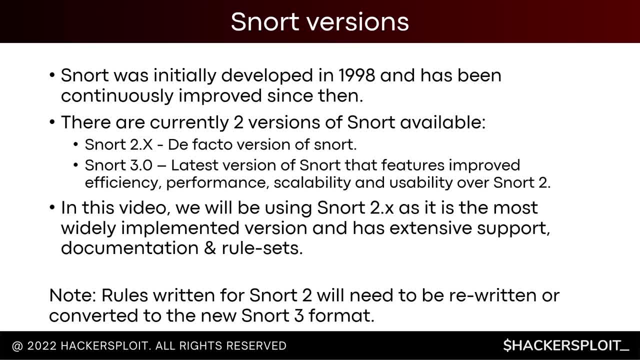 efficiency, performance, scalability and usability over snot 2.. not to say that snot 2 is slow, sluggish or, you know, does not offer any good usability or scalability functionality. it's just an improvement on top of snot 2.. in this video, we will be using snot 2 as it is the most widely. 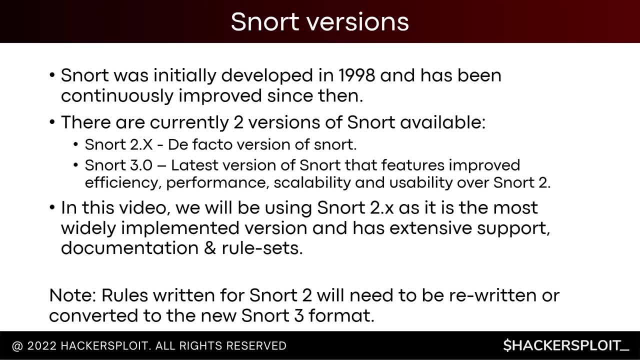 implemented version and has extensive support and rule sets created by the community. one thing to note is that eventually we will be migrating to version 3 and version 2 might as well be deprecated. however, i do not see that for the foreseeable future because, as i said, one of the issues that snot has faced is the 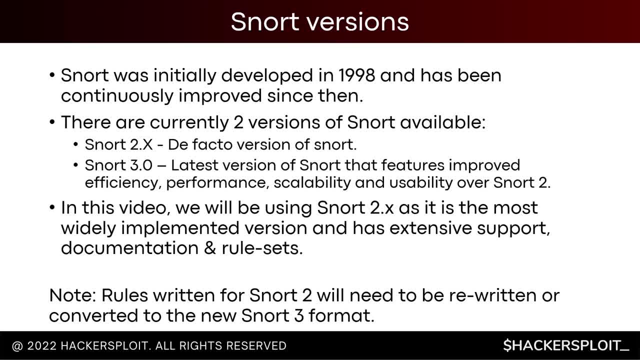 fact that when they released version 2, that version was. you know that that's essentially when when snot started becoming mainstream and a huge number of their customers- or you know, users who use snot- are on version 2 and in order to migrate to version 3, there are 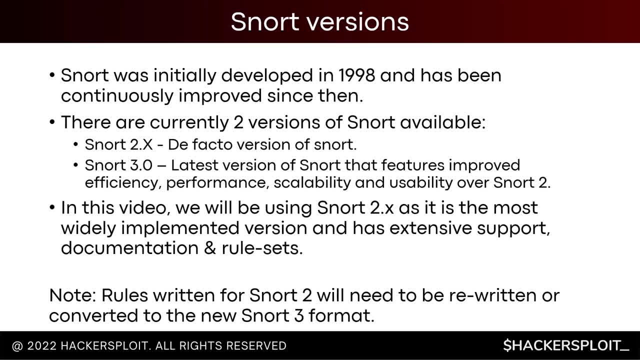 a few things you need to take into consideration, the most important of which is the actual rule format or the actual syntax for for writing rules whereby rules written for snot 2 will need to be rewritten or converted to the new snot 3 format and, of course, in the case of snot 3. 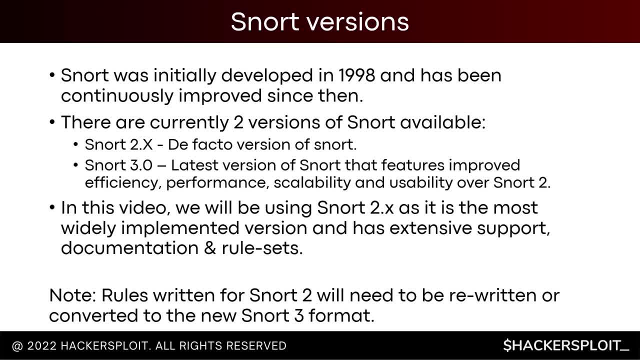 the snot configuration file is programmed in the lua programming language, so there's a lot of changes, and the reason i'm focusing on version 2 is primarily because this is the easiest and best way to actually get started with understanding snot- uh, learning how to use it, and 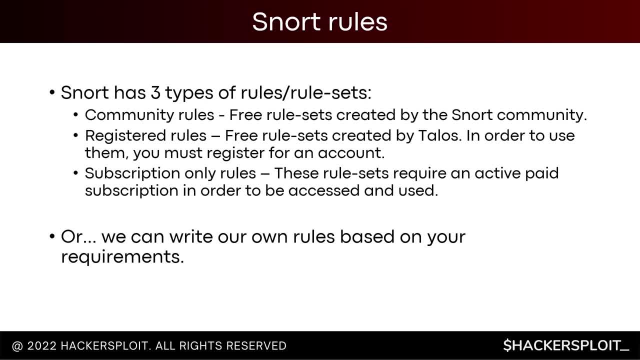 of course, implementing it within your own network. now let's talk a little bit about- uh, you know the snot rules because i've mentioned them quite a bit. so snot has three types of rules or rule sets. you have your community rules, which are free rule sets created by the snot community. you have 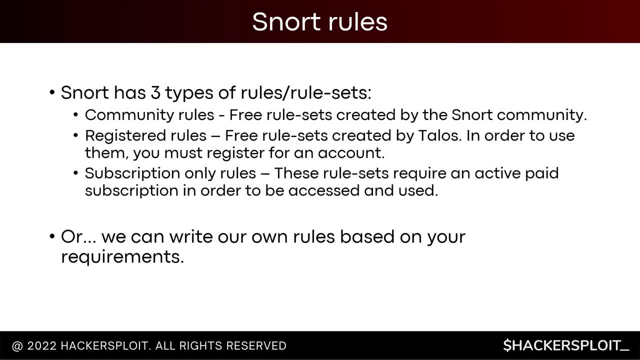 rules: these are free rule sets created by telos in. in order to use them, you must register for an account. they're very useful and then, of course, you have your subscription. only rules: these are rule sets. uh, these rule sets require an active paid subscription in order to be accessed, and 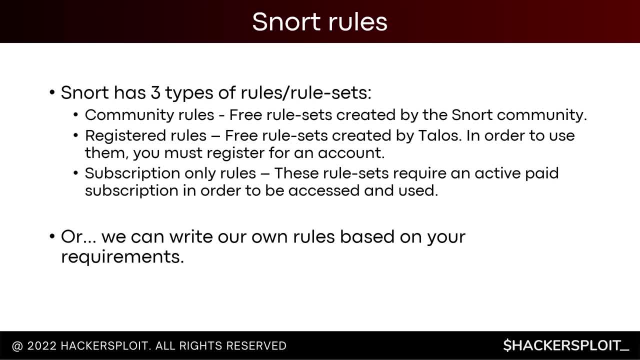 used. so i think it's about 39 per month that you pay to snot, and this is very useful for companies whereby you're essentially outsourcing your threat intelligence to snot and there, and you know, based on that, you can write your own rules based on your own requirements. right, and then, if you're 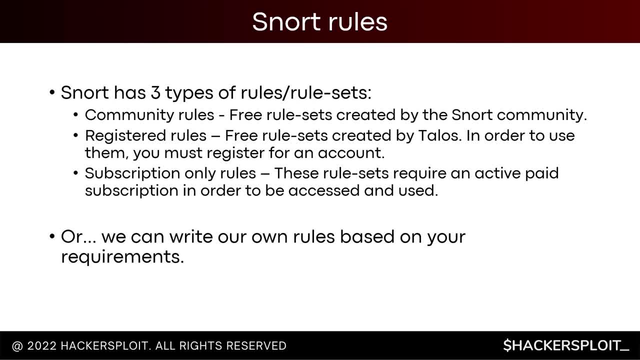 on a snot cloud or you're on a mobile phone or you're on a tablet and you have a snot. you can go through and, uh, use the snot rules. you can go through and download these rule sets and deal with the power of snot, and i'll talk a little bit more about snot rule sets in a bit. 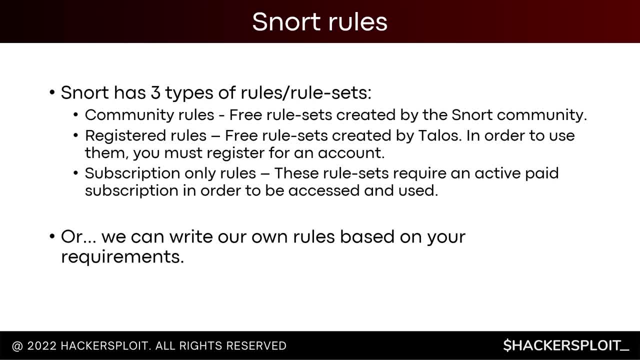 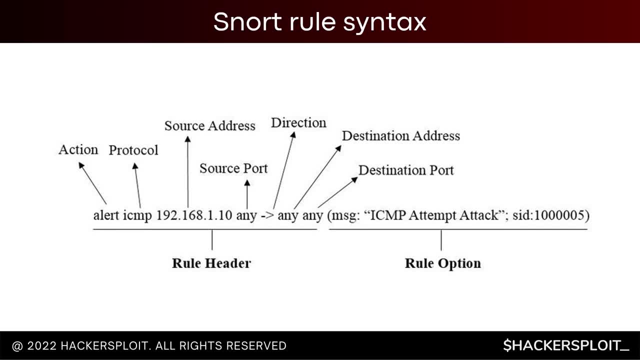 but first of all, just make sure that you've got a snot rule set so that you can use it when you're working or when you're not working, and that's a really great way to build up the skills you have and that's a really great way to develop a snot rule routine. 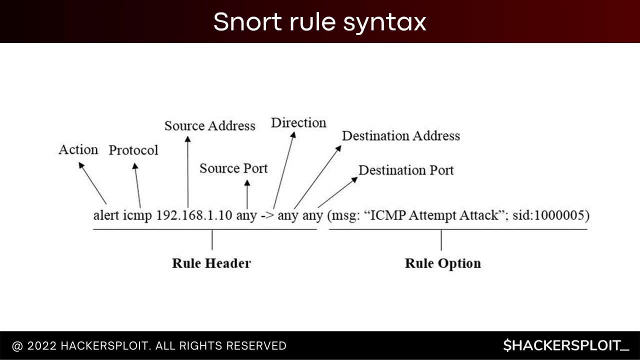 it's very important that you understand the syntax. As I said, it's very easy. Once you start writing rules yourself, it really is very easy. So the first, the first segment here, and this is typically separated with this direction. So that's a hyphen and greater than. 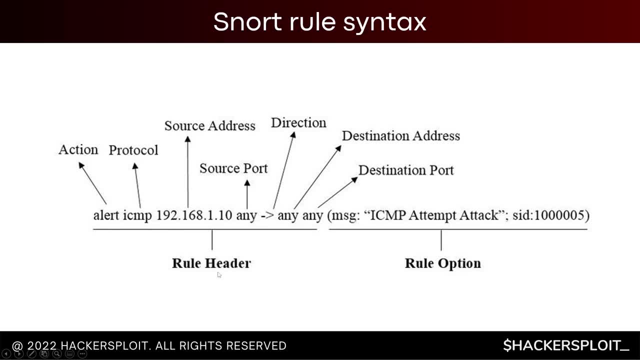 symbol. So this is where you specify the rule header right, and then you have the rule options. So this is the rule header, And then you're going to say: you know, you're going to specify options pertinent to that rule. So in this case the action is alert. So that means that in the case 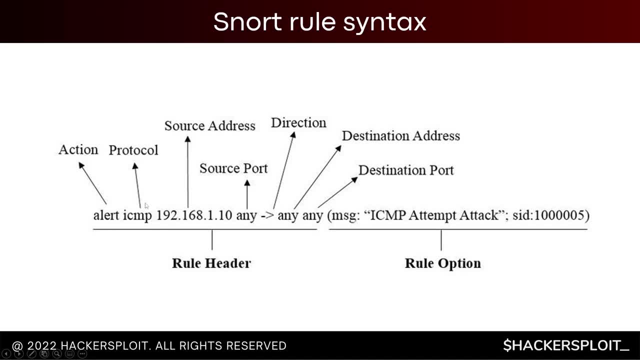 of this rule. when there is an ICMP packet or ICMP traffic coming from the following IP address: from any port to any, to any IP address and any port on the target network or the network that you are protecting or that you have snort configured to monitor, then log the following: So the message: 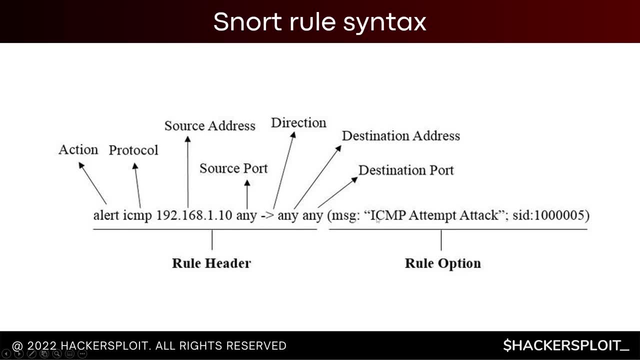 is going to be: or send the following alert and the message is going to be: ICMP attempt attack. And then it has a signature ID which you can essentially, you know, create your own signature IDs based on your own requirements. So it really is very simple. So you're essentially saying: 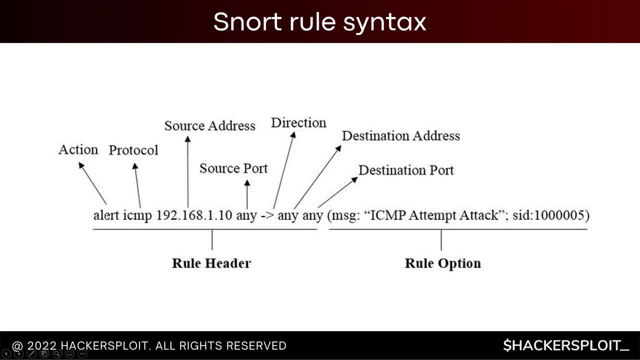 the action firstly, which can be alert, drop log, you know, etc. etc. And then the protocol can be ICMP, TCP, UDP, IP, etc. And then you can specify the source, the source IP address, And in this 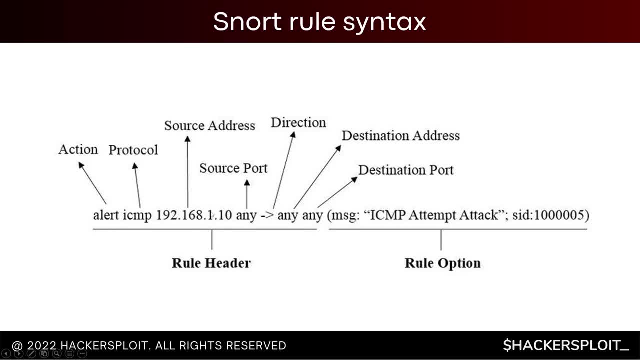 case you can also say So. you can say any traffic coming from any IP address, from any port that comes into our home network, which I'll explain. on a specific port or on any port, you then, you know, essentially specify the rule option. it's really very easy. This will make sense once we get into the practical. 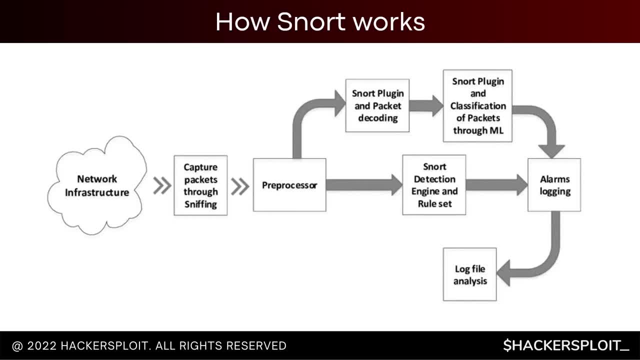 demonstration: iencia. So how does snot work, Right? So this diagram really explains what happens, right? So you have your network infrastructure and then in the port, here at the base, we have a digital database. Okay, incoming traffic comes into the SNORT host or the SNORT server, and then you can see right over here. 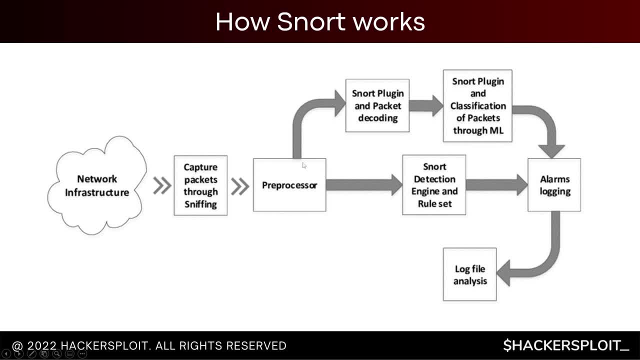 capture packets through sniffing, so it captures all the packets for all the devices or hosts on the network. it then goes through a pre-processor and then it goes through the SNORT plugin and packet decoding and then, of course, it goes through the classification of the packets and, in the event, 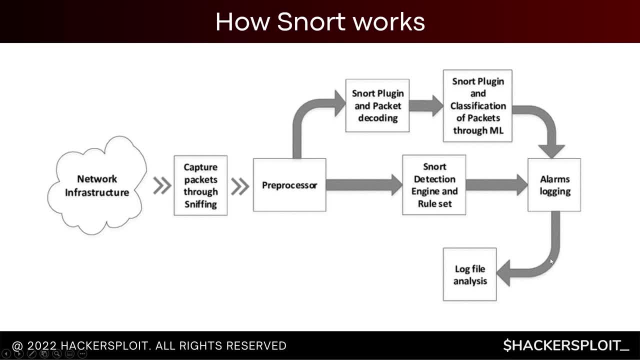 a signature is matched. alarms: the alarm logging process is essentially implemented where it's either logged or an alert is sent and you know it also goes through the SNORT detection engine and rule set and again that all comes into the alarms and logging process or segment. you know. 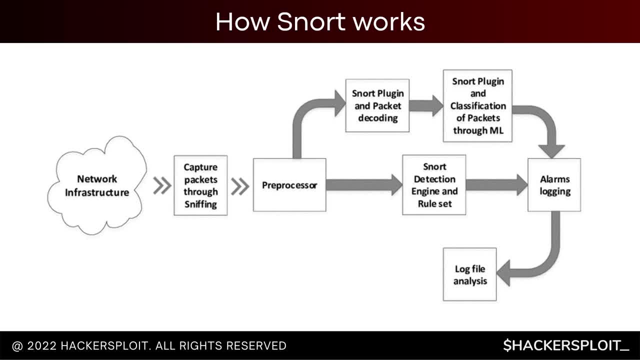 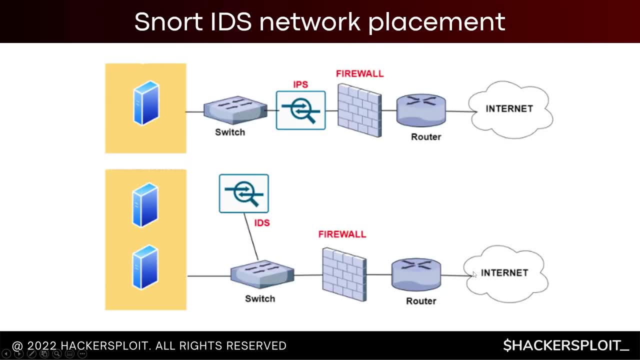 in regards to how SNORT processes or essentially handles traffic, and then, of course, you know, it goes into a log file for analysis. Now, this is very important because I do know that this can be quite confusing. As I said, SNORT can work in a lot of different ways and I'm going to show you. 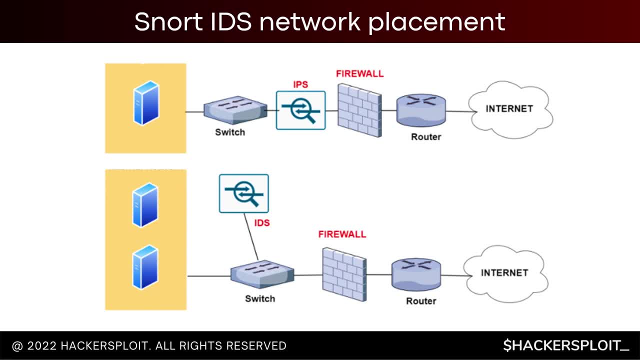 how it can work in two modes, and this is very important, right. it can work as an, as an intrusion detection system or an intrusion prevention system. Now, in this, in these, in this particular diagram, you have two use cases. the top one is for is, whereby you can use SNORT as an intrusion. 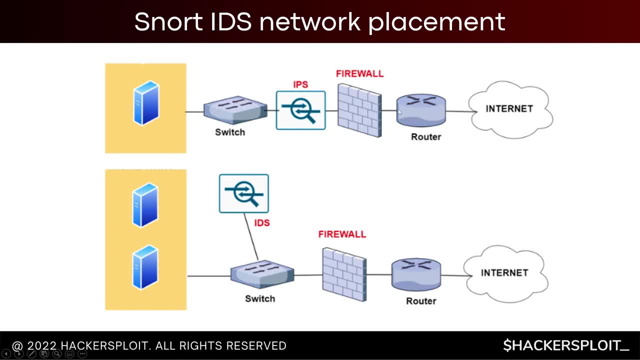 prevention system. so you have your internet, you have your router and in some cases you may have a firewall, but you can disregard that. so ideally you want to use SNORT as an intrusion prevention system because you want to place the system that is running SNORT between the router and the switch. 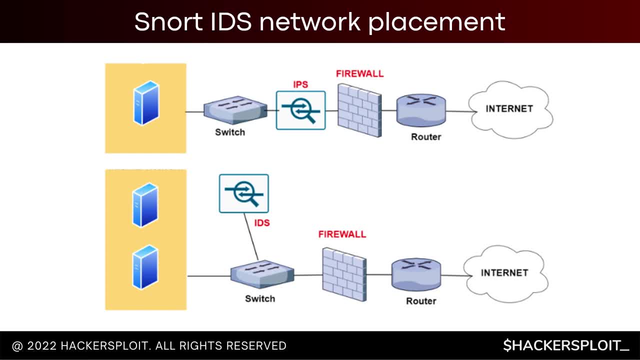 so remember: all traffic. that means that all traffic is is coming in through SNORT and it also goes out through SNORT, right? so you want, in the case of an intrusion prevention system, or whereby you want to use SNORT for intrusion prevention, then you want to set it up at a choke point, right? 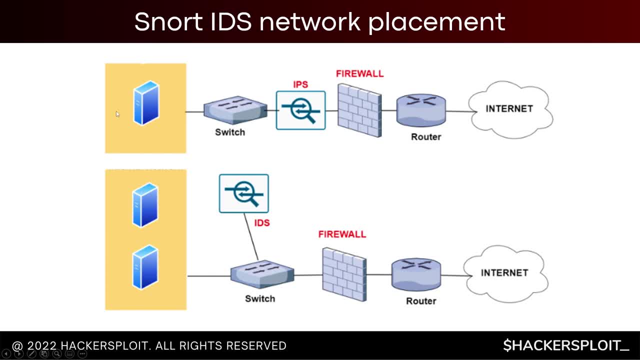 and you know that's fairly simple to understand. so that means that any any communication coming into any of these devices within your network, your internal network, are all going through SNORT, and you know it can then decide to drop packets based on the rules that you specify now, if you want to use it as an intrusion detection system, which is what we are. 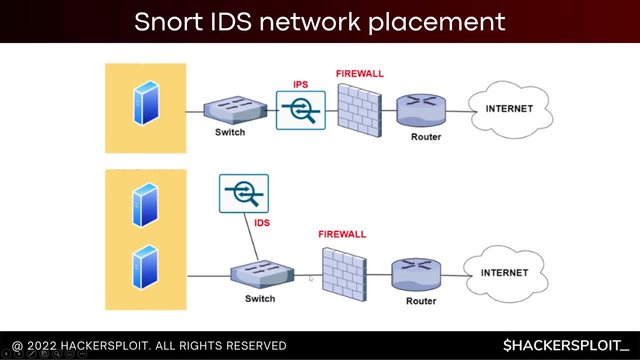 going to do. you can see, you have the internet, you have your router, a firewall. you're essentially connecting it to a switch. so if you're on a LAN or if you're using a virtualized environment, like you know, like with VirtualBox, then the switch aspect is already taken care for you. so if you have more than one virtual machine, 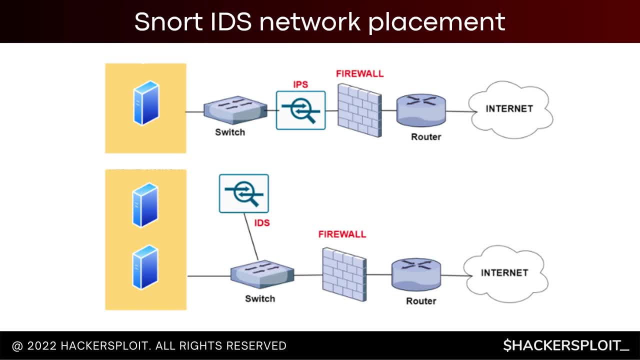 connected to the same type of network adapter, then they're going to be connected to each other through a virtual switch. so ideally you want to have your the- the actual server running SNORT- connected, or part of the network that all the other VMs are a part of, which is what we're going. 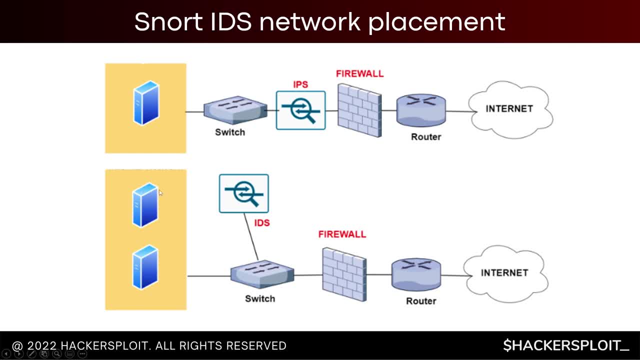 to be doing so. ideally this should fit within that network, so they're going to be on the same subnet but they're all connected to the switch. so that means that you know SNORT is essentially monitoring all traffic that is coming in and out. of. you know all the devices on the network and 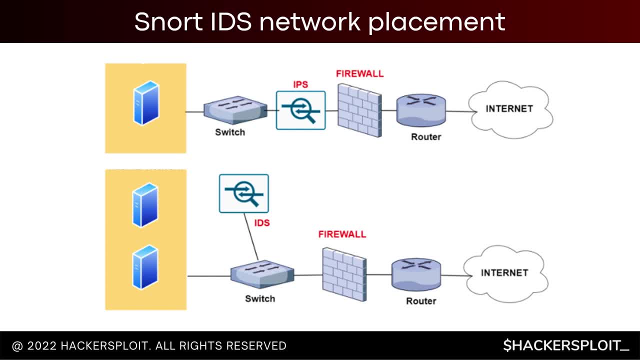 based on that traffic. it, you know, tells you what's happening. so it'll tell you, you know, based on your rules, whether there's an intrusion, whether you know a ping has been performed, etc. etc. so there's multiple ways of configuring it and, as I, as I would say, if you are looking at implementing, 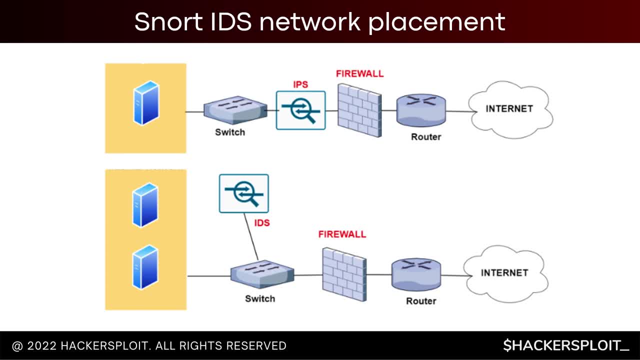 a system, then this would best be implemented within a physical network, within a real network, as opposed to a virtualized environment. however, in our case, because I need to showcase this, you know, I need to actually showcase how to use SNORT as an IDS. we'll be doing it through VirtualBox. 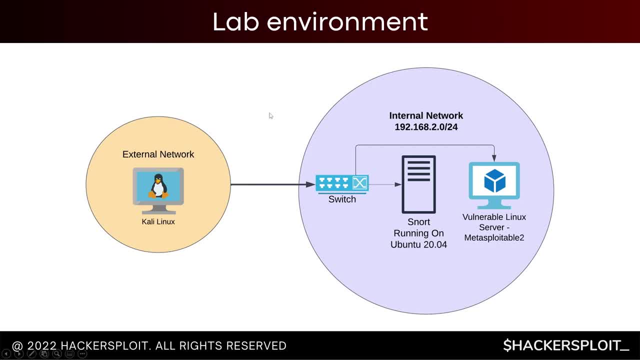 all right. so this is the lab environment. it's fairly simple. so we are going to have an external network, so this is where we're going to have the Kali Linux virtual machine. so this is running on another network adapter, so this is running on a NAT network. and then, of course, we have the following segment, which is the 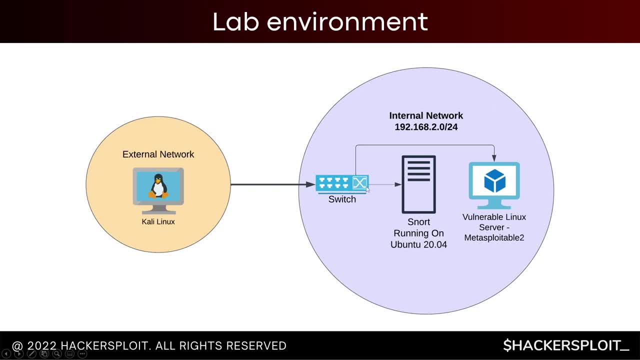 internal network whereby we're going to have the VirtualBox switch here, and you can see that in this case the subnet is 192.168.2.0 forward slash 24. in your case it's going to be different. ideally, what I'm saying is all of these three systems: the Kali Linux VM, the Ubuntu 20.04 VM running SNORT, and 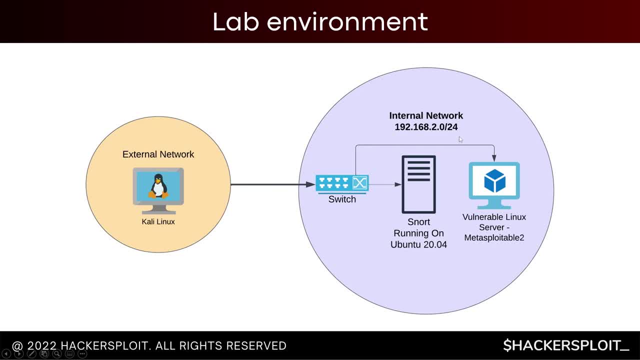 the Vulnerable Linux Server are all running on VirtualBox. however, these two are running on the same network, on or on the same network adapter, and this one is running on a different network. right in order to simulate what would happen if external traffic, you know if there was traffic from an. 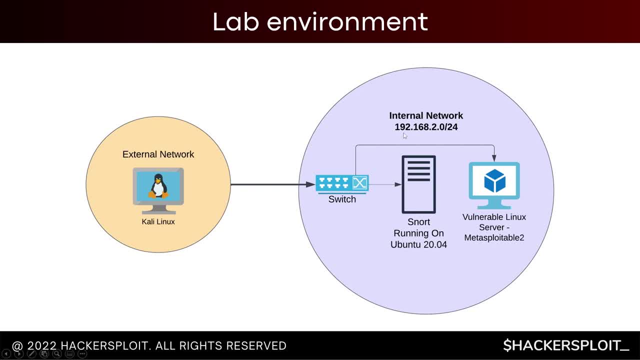 external system and, of course, you can also have this within the same internal network because, again, remember, we're essentially monitoring the traffic for our current, or for you know, for the current- VMs, and this will be a test run of these three VMs. but, once again, this is going to be the